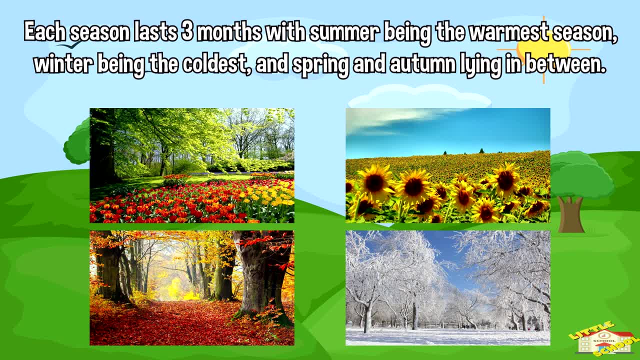 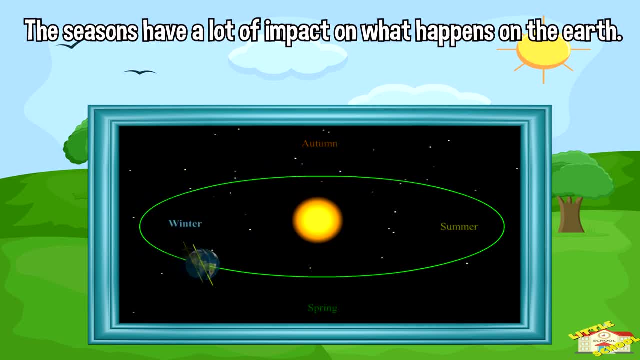 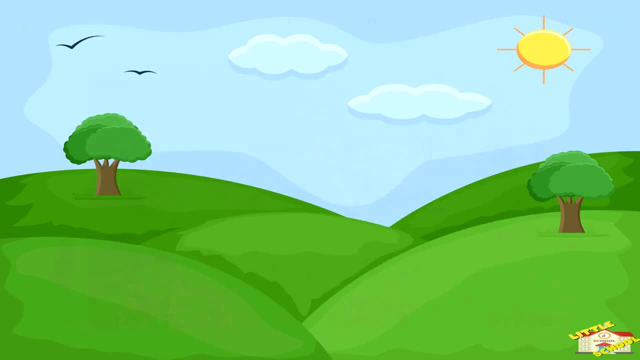 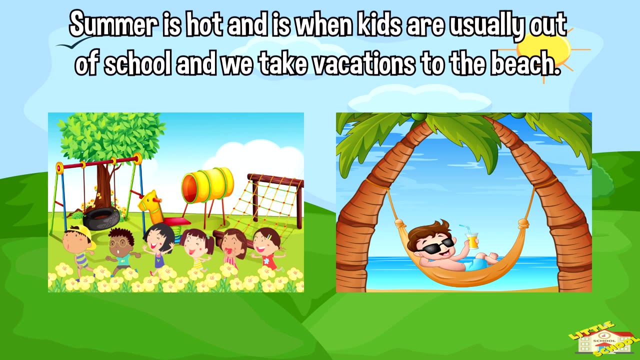 and autumn, lying in between The seasons, have a lot of impact on what happens on earth. In the spring, animals are born and plants come back to life. Summer is hot and is when kids are usually out of school and we take vacations to the beach. Often crops are harvested. 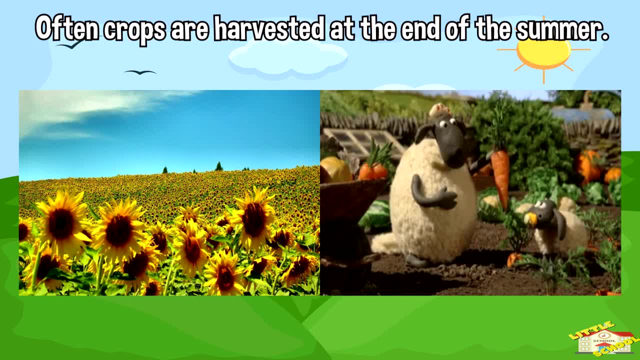 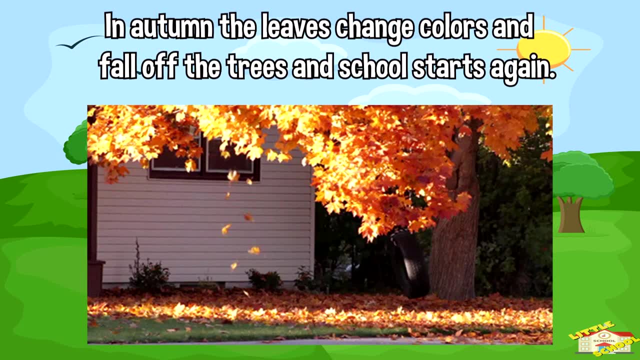 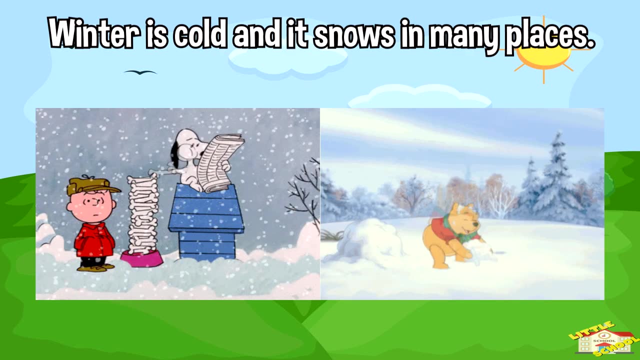 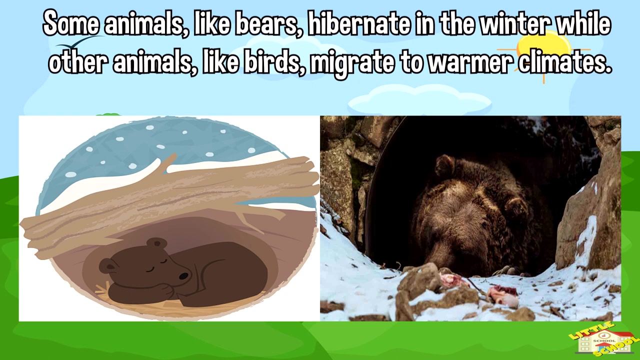 at the end of the summer. In autumn the leaves change color and fall of the trees, and school starts again. Winter is cold and it snows in many places. Some animals, like bears, hibernate in the winter, while other animals, like birds, migrate to warmer climates. 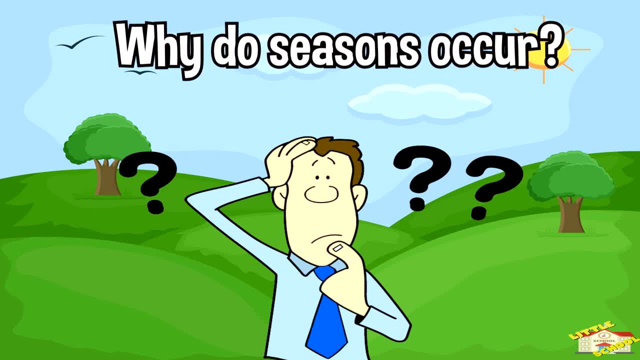 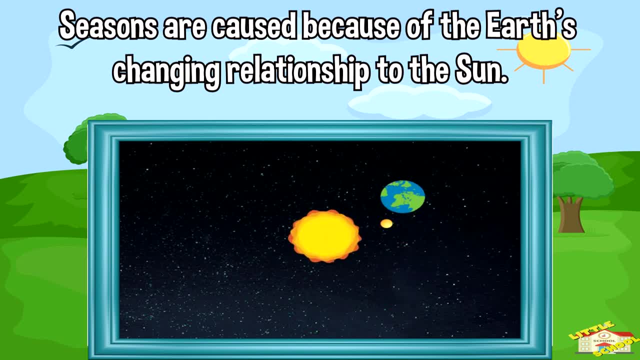 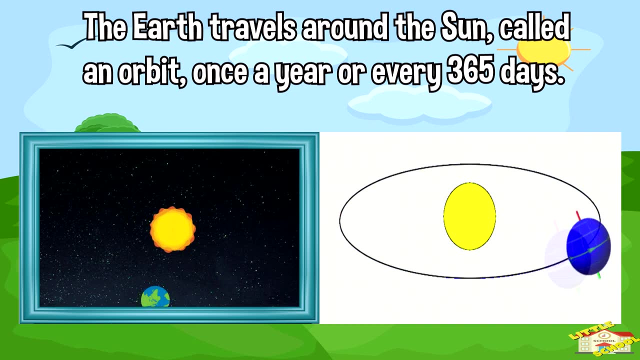 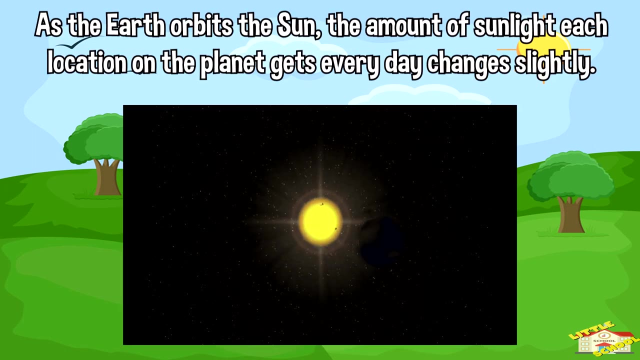 Why do seasons occur? Seasons are caused because of the earth's changing relationship to the sun. The earth travels around the sun, called an orbit, once a year or every 365 days, As the earth orbits the sun. the amount of sunlight each location on the planet gets every day. 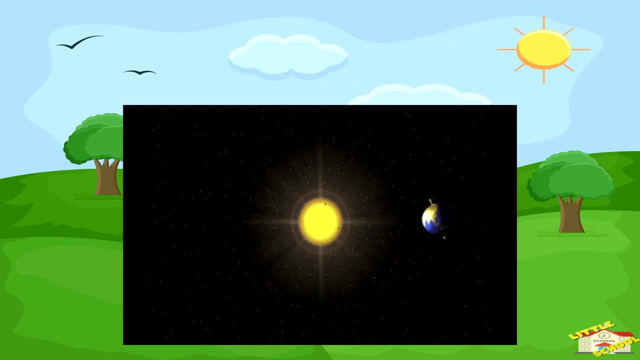 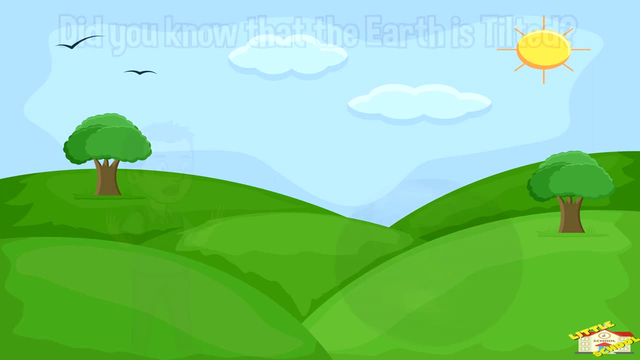 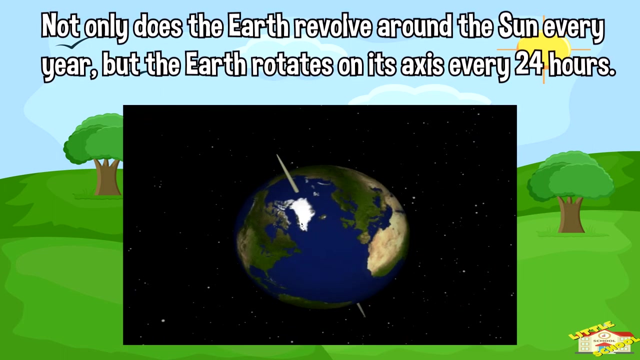 changes slightly. This change causes the seasons. Why do seasons occur? 1., 2., 3., 4., 5., 6., 7., 8., 9., 10., 11., 12., 13.. 14., 15., 16., 17., 18., 19., 20., 21., 22., 23., 24., 25., 26., 27., 28., 29., 30.. 31., 32., 32., 33., 34., 35., 36., 37., 38., 39., 40., 41., 42., 43., 44., 44., 45.. 46., 46., 47., 48., 49., 49., 50., 51., 52., 53., 52., 53., 54., 55., 56., 57., 58.. 59., 60., 61., 62., 62., 63., 64., 65., 66., 67., 68., 69., 69., 70., 71., 72., 72.. 73., 74., 75., 76., 77., 78., 79., 80., 80., 81., 82., 83., 84., 85., 86., 87., 88.. 89., 90., 91., 92., 92., 93., 93., 94., 95., 96., 97., 98., 99., 100., 100., 100. 100.. 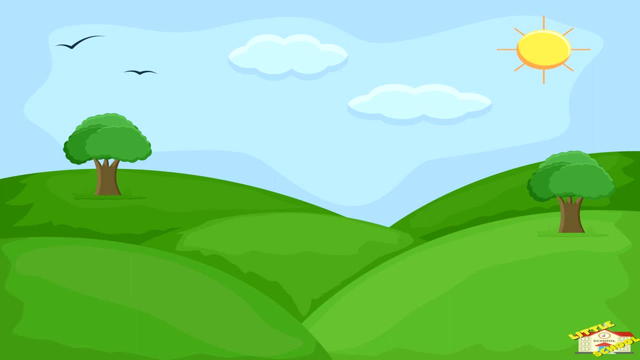 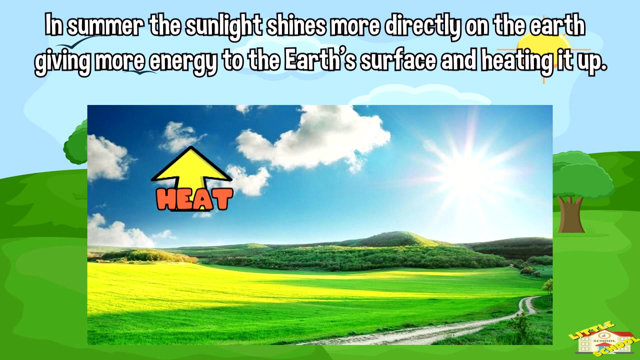